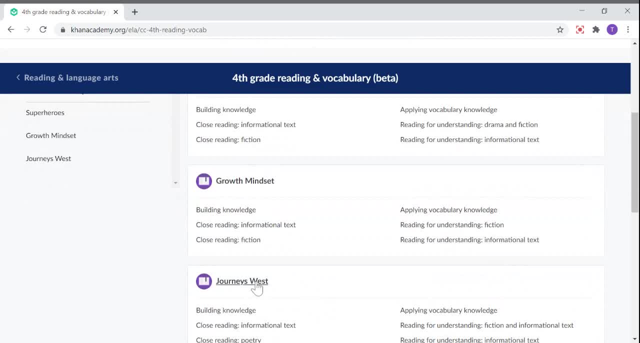 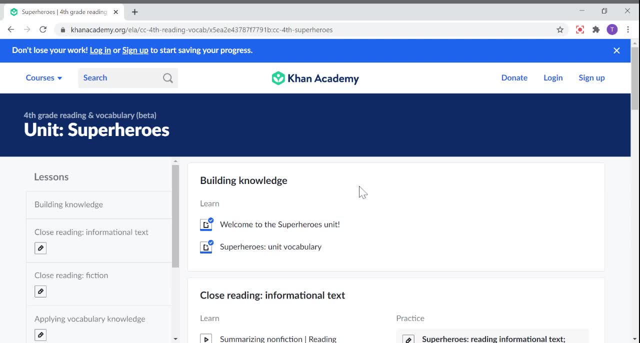 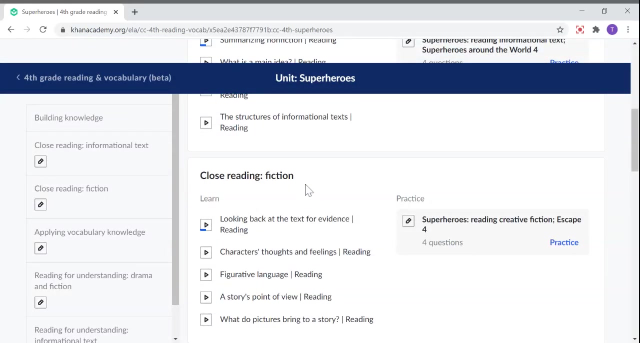 superheroes growth mindset and journeys west. Let's check out the superheroes unit and see what it's all about. Okay, so we've got some different lessons here, or different sections to this unit. First one is building knowledge. We've got close reading, informational text, Close reading for fiction, So your student is learning. two: 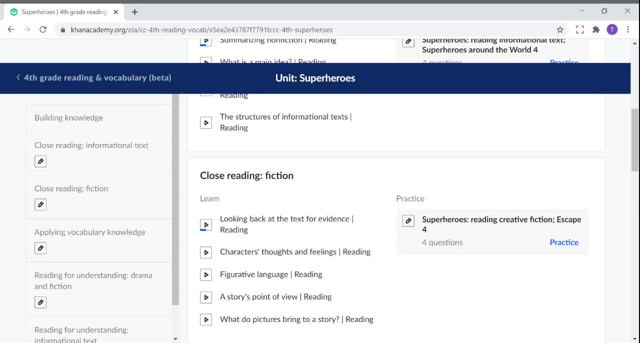 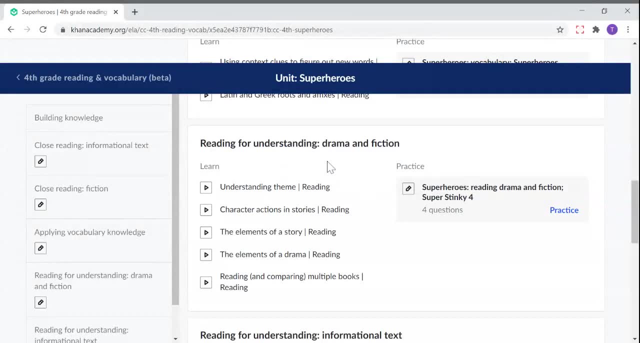 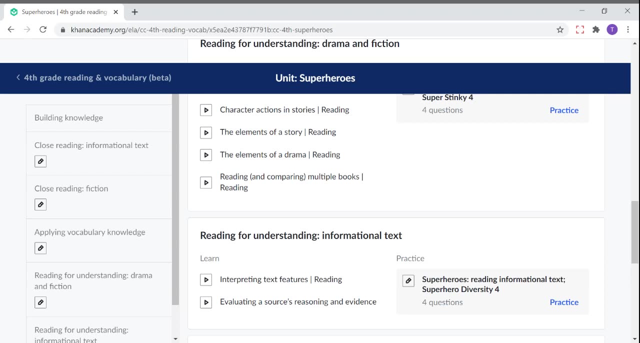 different skills here, or a skill for different types of writing. Very valuable. Then they're applying vocabulary knowledge and reading for understanding with drama and fiction, reading for understanding with informational text. So again, that's reading, comprehension, but for two different types of writing. Very useful stuff. 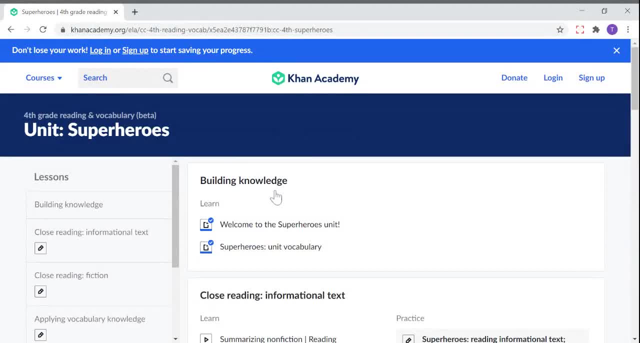 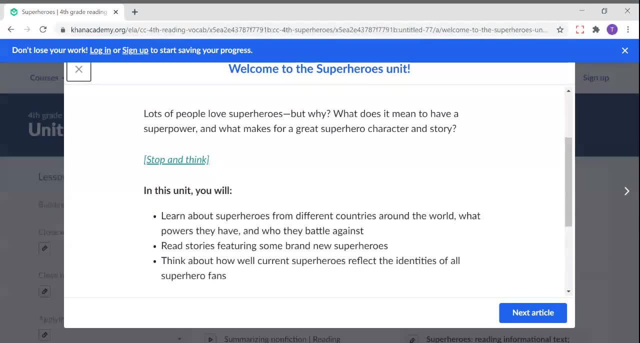 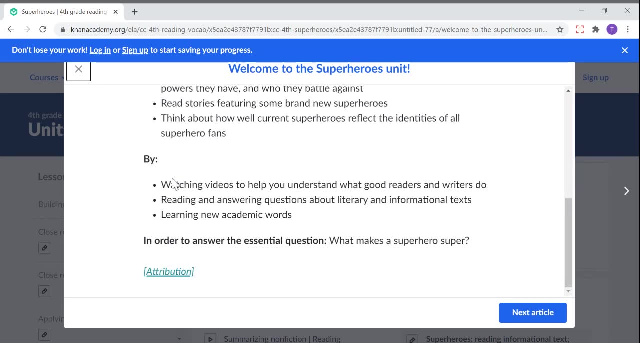 Okay, So let's start out with building knowledge. This is sort of an introduction to the unit. So we've got a welcome to the superheroes unit And it tells us about what the students will be doing here so they can anticipate their learning. Tells the students or you how they will be doing that learning watching. 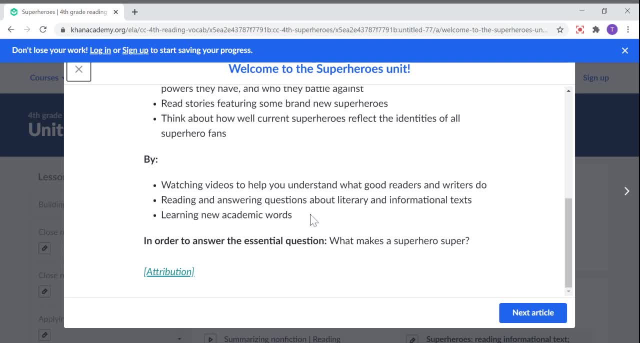 videos, answering questions, learning new words, And a nice thing here is it's got an essential question here. That's always a great way to frame learning If we are always keeping in mind what makes a superhero, if that's sort of the theme question for our learning. 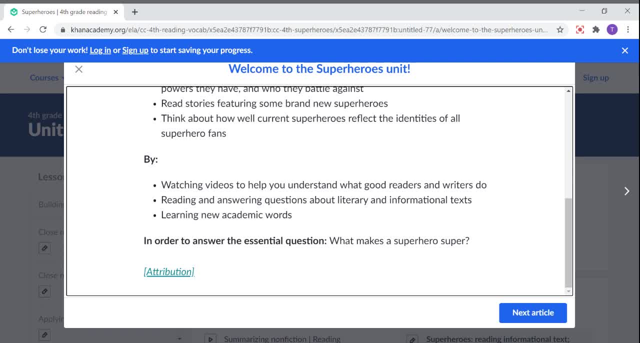 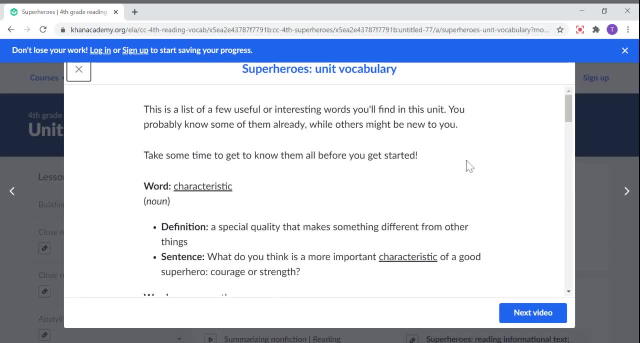 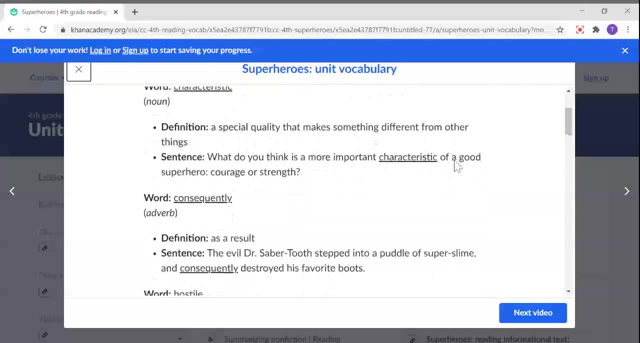 then we can keep referring back to that and adding to the answer for that question as we learn more. Okay, Now we have some vocabulary that the students can learn. It's always a great idea to learn vocabulary beforehand. That way they're more likely to understand what they're reading. 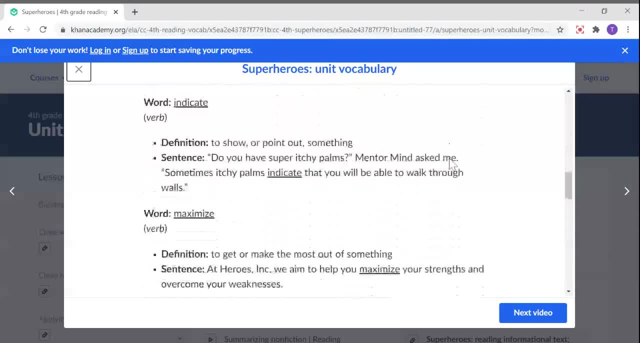 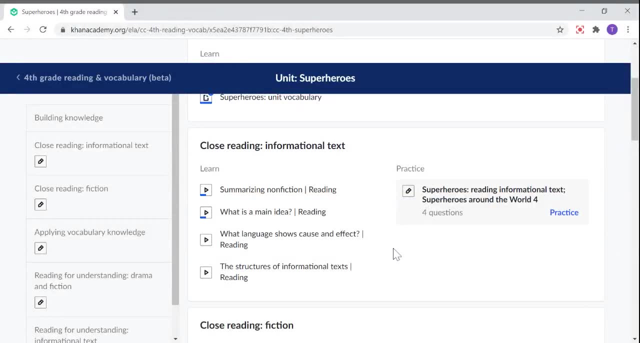 as they are going through it. So we've got a handful of vocabulary words here, Great way to start. And then let's look at our first lesson, or the first part of this unit here. So this is close reading for informational text, And these are four videos that are going to. 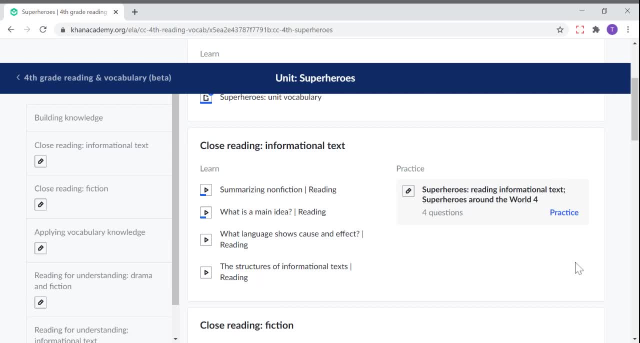 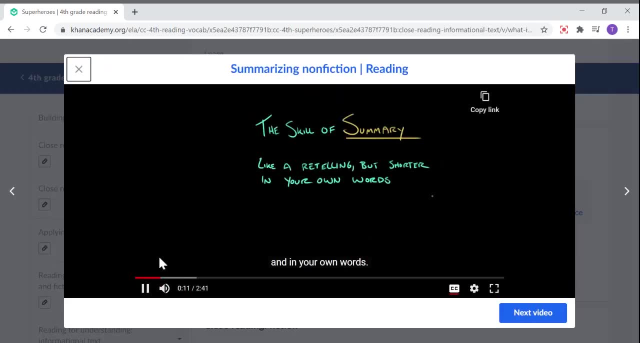 do some teaching so that our students can learn, And then they'll practice applying their learning with this section here. So let's check it out, This first video. We want to start with the foundation. Okay, So this video is teaching our students about summaries. It started part way through. 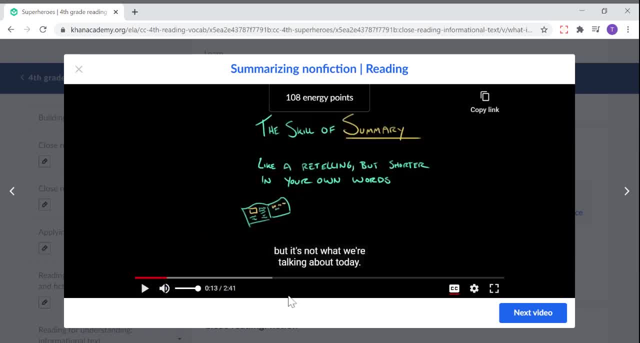 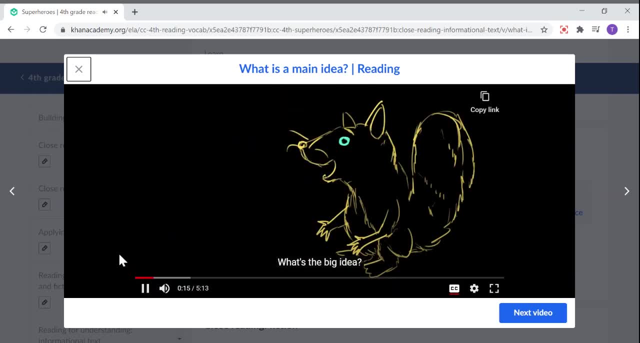 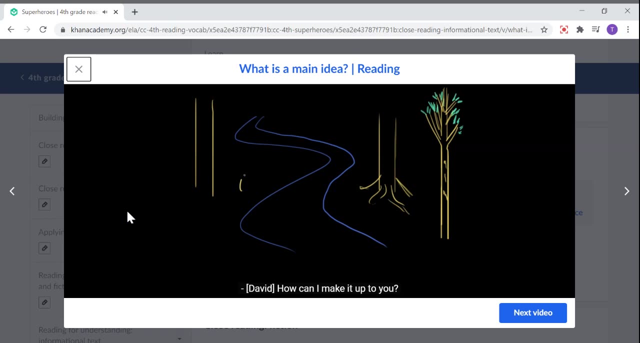 because I've started watching it before. But let's see what our next video is about here. Great for advanced readers. So we want to start in one sentence. So here's another fun video, and again it started part way through because I've been 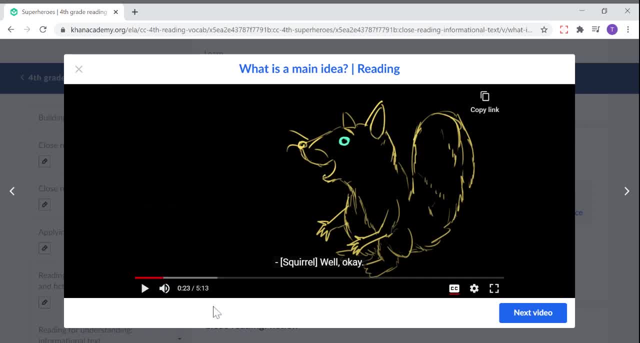 watching it already, But these are great videos. they're not terribly long- this one's five minutes, and usually they're between three to five minutes- and that's great because they're more likely to hold our learner's attention for that shorter time span. 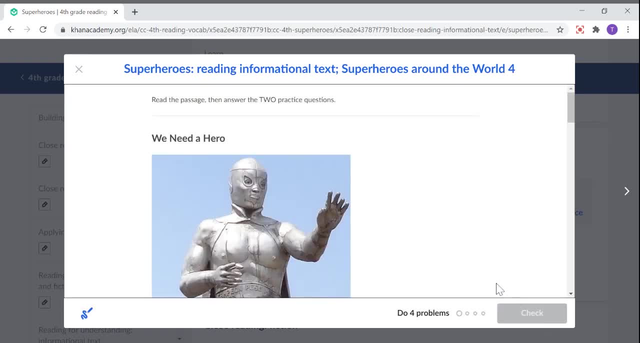 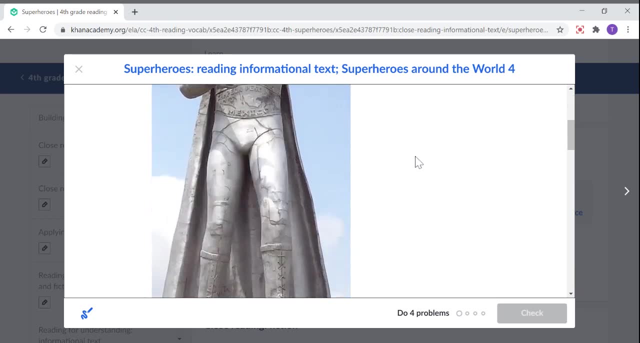 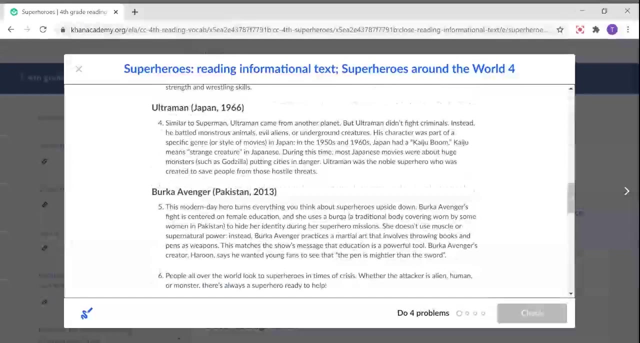 And then we can check out the practice here. So with the practice we've got instructions. read the passage, then answer the two practice questions. there's some reading here about different superheroes from different countries or different cultures, and then practice questions. 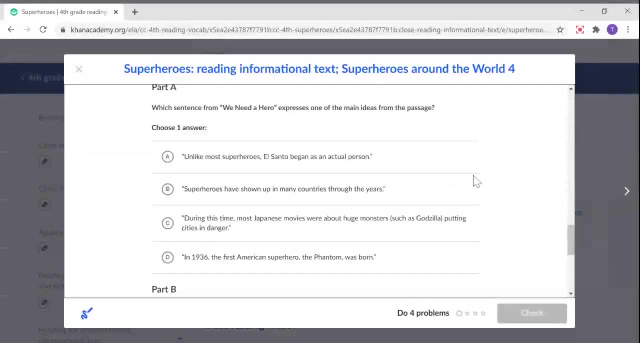 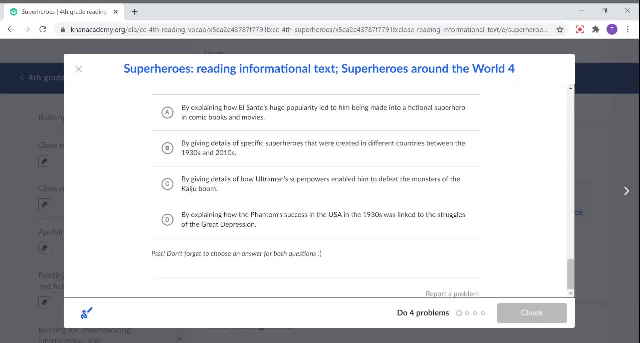 This question has two parts: answer part A, then part B. so the student is going to need to choose one answer here, one answer there and then they can check their answer and there are four different questions or four sections for them to go through to practice their learning. 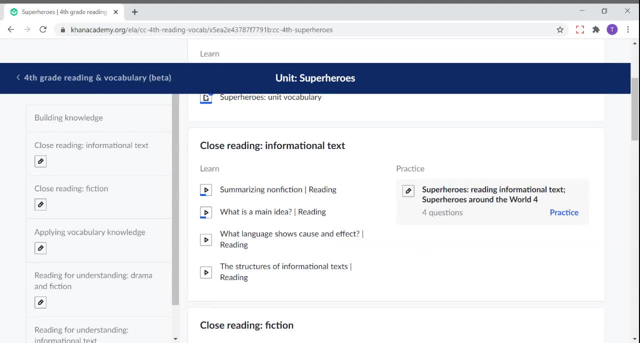 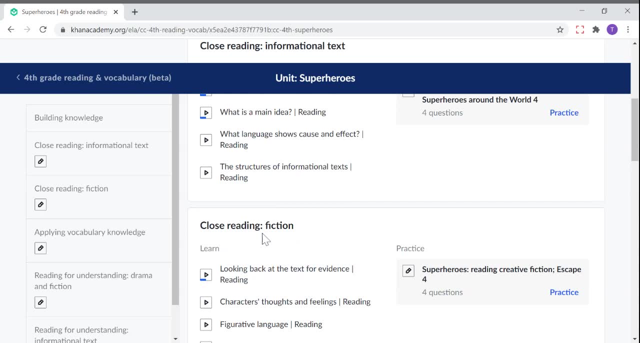 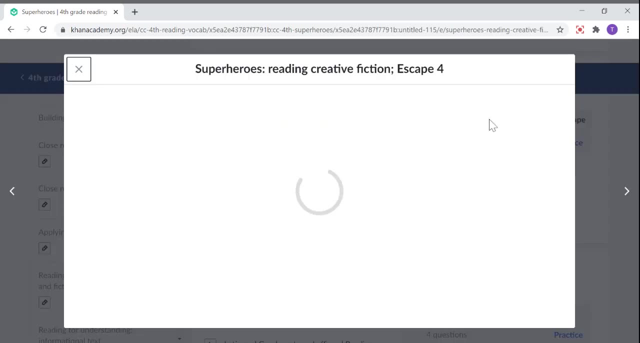 So this is a really great video. It's a great skill for them or a great way for them to learn about reading informational texts or non-fiction texts. We've got fiction reading here. these are all videos, but let's see what other reading. 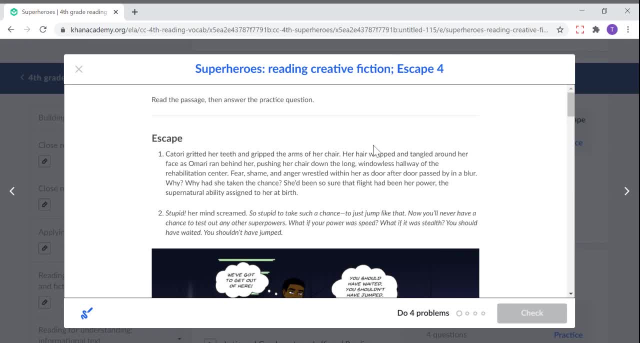 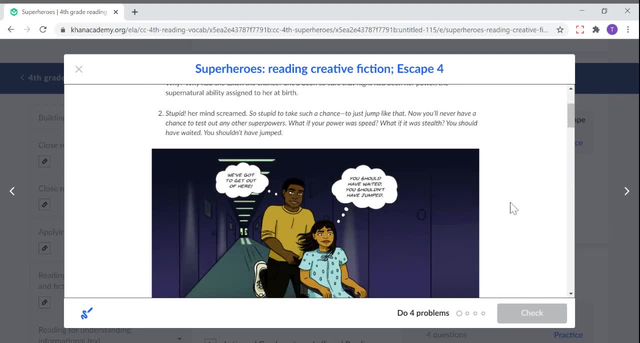 we've got here for them to practice, Okay, so we're going to read the passage and then answer the practice question. So we've got a nice combination here of videos where they're listening, They're reading and having a visual to understand and do some reading that way. 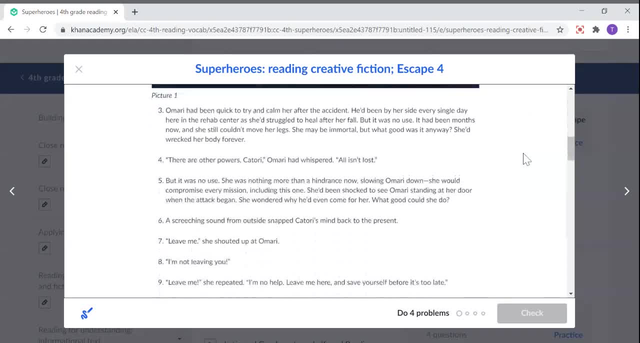 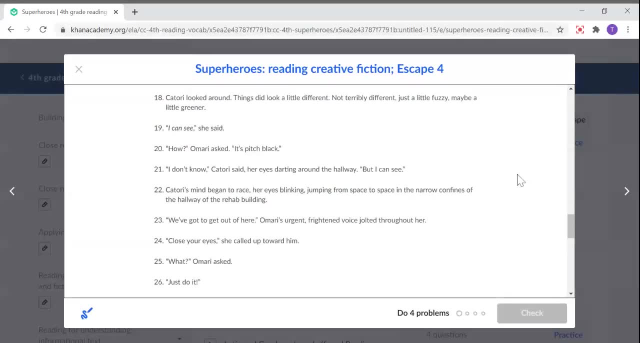 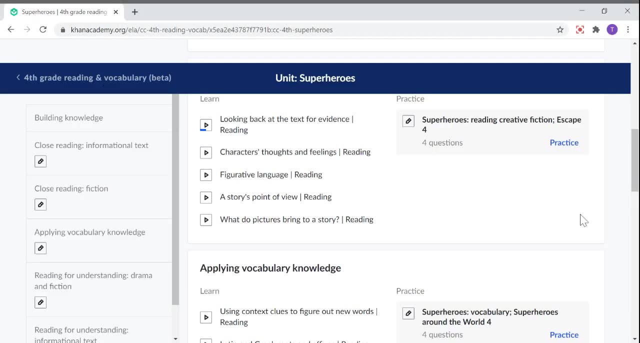 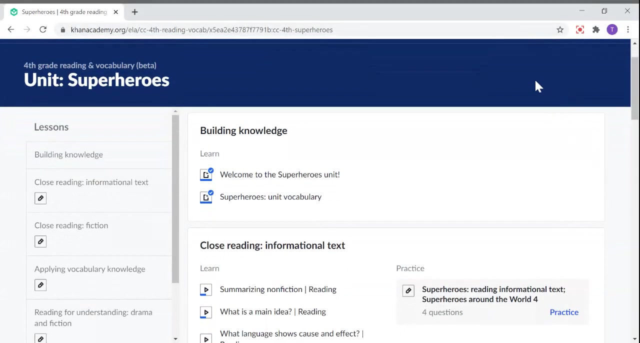 And then these readings require them to read through, and then it checks their understanding of what they've read- Great stuff. Now, one thing to remember is that this is from the US, so it's based on American grade levels and American curriculum content, But it's still really valuable for us Canadians.